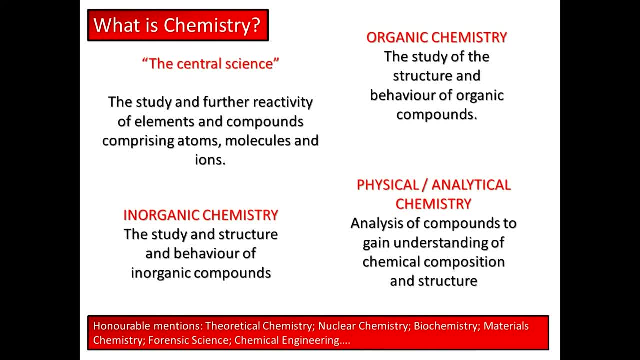 things such as theoretical chemistry, nuclear chemistry, biochemistry, materials chemistry, of course, forensic science and chemical engineering, both subjects that we do offer at the University of Wolverhampton as well. So it's a huge area and it does split into roughly three different areas. However, these areas, as you'll find out over the years, 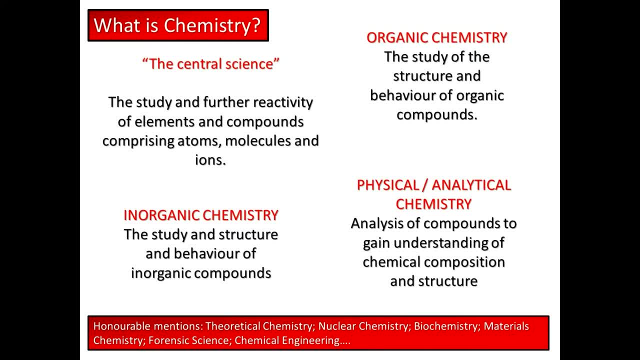 if you do start to study chemistry, they merge into one big kind of area called chemistry. so first of all, organic chemistry is essentially the study and structure and behavior of organic compounds, and I'm going to discuss what organic compounds mean very soon. Inorganic chemistry is: 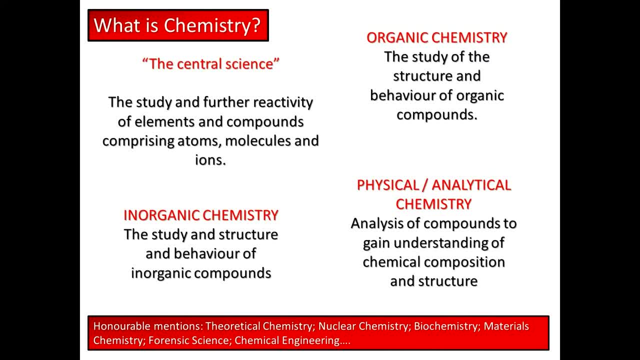 of course, the study and structure of inorganic compounds. So, essentially, what chemists tend to do is make new materials, albeit they may be inorganic materials, they may be organic materials. but we tend to make new materials and we make them for a reason. Of course they may have some. 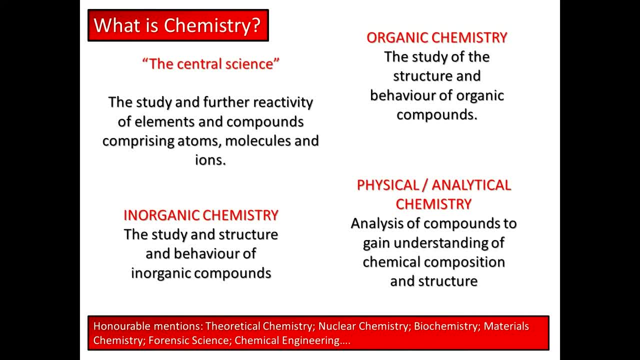 behaviour or an ability to do something that will help the public. Okay, for instance, once we've made these materials, of course we're going to have to work out whether they are actually useful or not, and, of course, this comes under the area of physical chemistry and analytical chemistry. 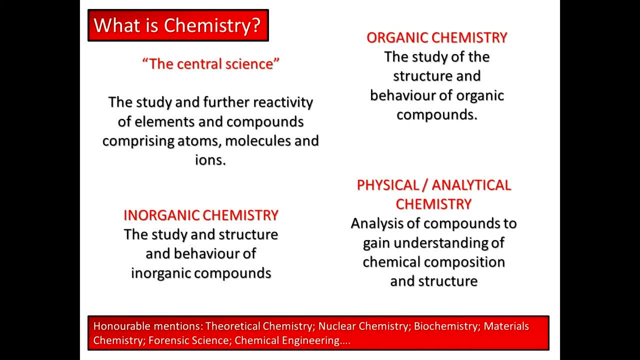 so, basically, the analysis of compounds to gain a further understanding of their chemical composition, their structure and, of course, to relate their physical properties with their ability to do things. So, for example, if you're looking at a chemical composition, you're going to have to. 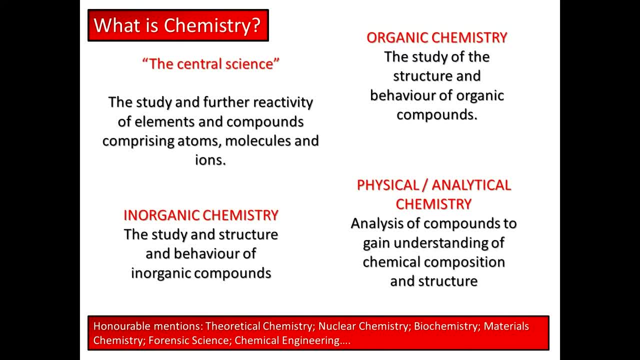 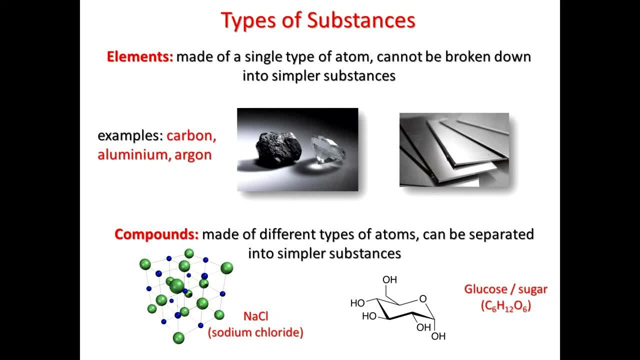 or applications. Okay, so it's a huge area. So, first of all, before we look at different types of inorganic and organic materials, essentially we just talk briefly about elements, of course, and these are found in the periodic table And of course, they're found in the ground and in the air. 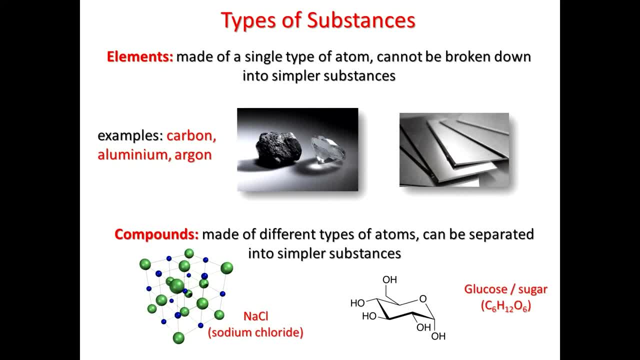 They're made up of single types of atoms and they can't be broken down into simpler substances In real life. of course they don't exist as single atoms. they are bound together through chemical bonding. I do have a chemical bonding presentation for you in this Aspire to HE. 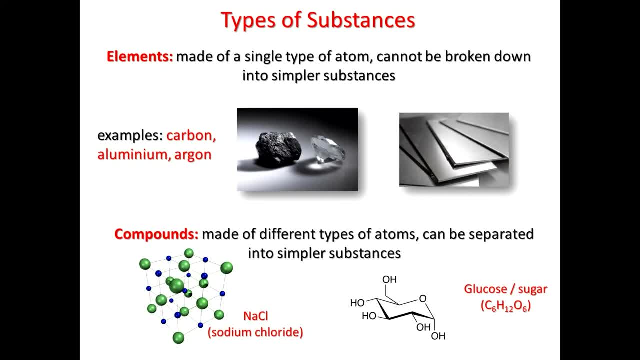 collaboration also, and that will be uploaded soon, But essentially. for instance, if you look at the picture on the top left, here you've got carbon and you've got two different types of carbon. So you've got diamond on the right, of course nice and clear and hard. Of course the 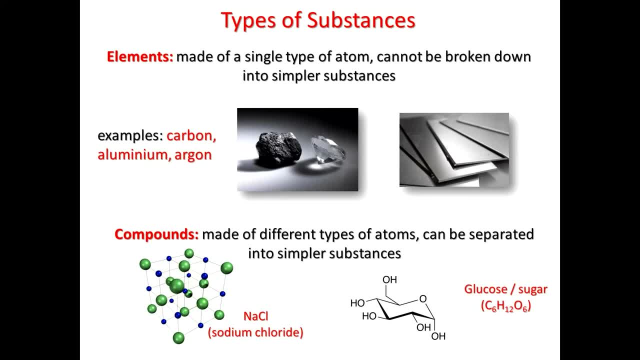 graphite, carbon or a piece of coal, essentially on the left, which of course has a much more sort of slippery and slippery kind of behaviour. Of course it's the reason that we use pencils, for instance, And on the right hand side, of course, we've got aluminium sheets which 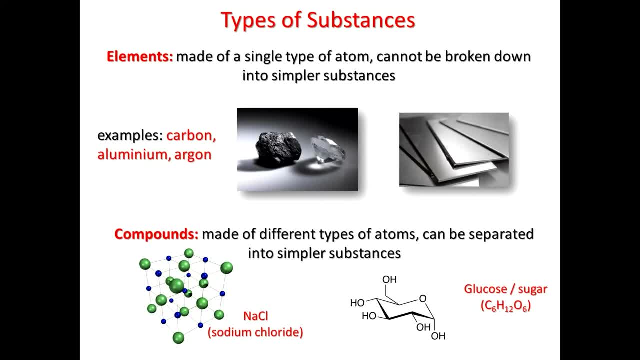 are just metals And, of course, that material is just made up of aluminium atoms linked together through what we call metallic bonding, And not pictured, of course, is perhaps argon gas, which is of course a gas, and so it's floating around us. in small amounts, However, we can actually 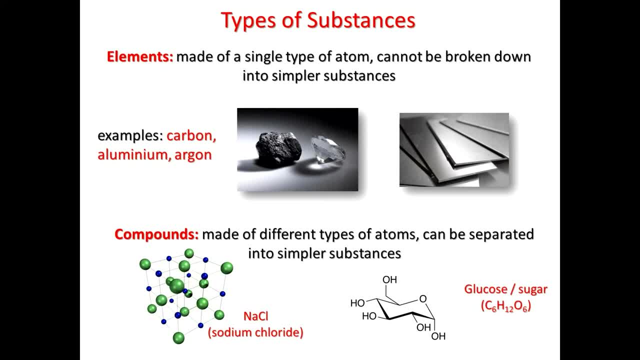 as chemists, and these materials are found in the ground and in the air also, but we can actually connect these different elements together to form interesting materials, So of course, some of them have been around for a long long time. of course, For instance, sodium chloride is what we call a. 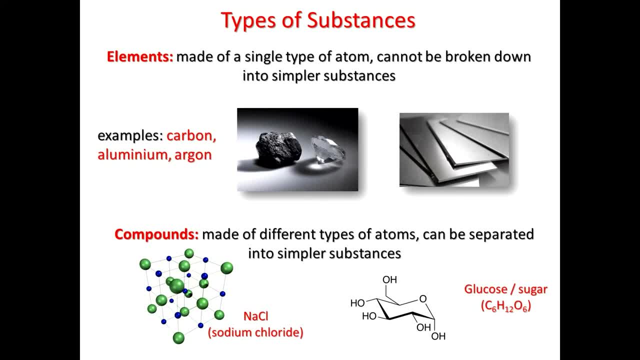 compound, and we call it an ionic compound. We do call it an inorganic compound as well, because it does not contain carbon, and we'll talk about that later, But essentially that contains sodium and chloride ions connected together. okay, to give you a compound, And this is, of course, table salt that we add to. 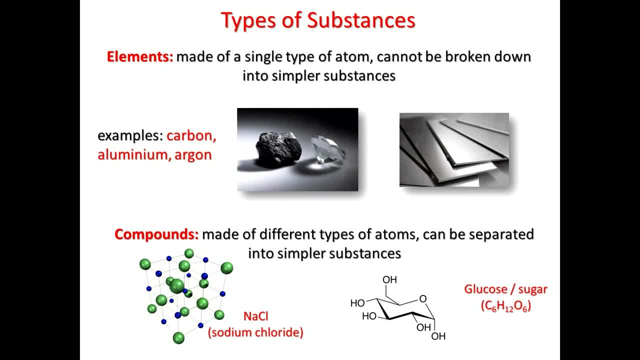 our foods and are found in nature, of course, in the sea, for instance, solubilized and slightly precipitous. If you connect a load of carbons and oxygens and hydrogens together in a ring-type structure, you'll notice that you can form a ring called glucose, and this is a sugar okay. 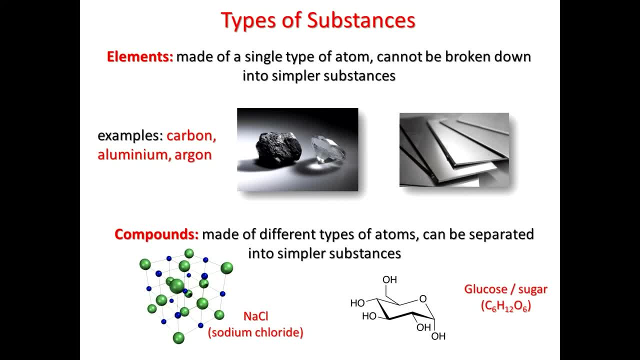 So essentially, just by combining carbons and protons and oxygens you can actually form sugar, which is a very, very important molecule. And of course there are many, many more examples of these in the literature and again found in the ground and synthesized in laboratories, and found in the air, et cetera. 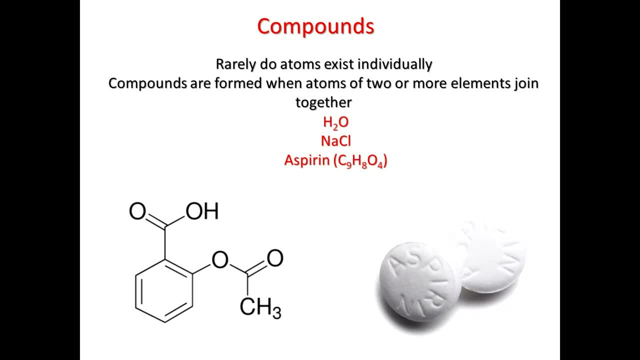 So, as I said, rarely atoms exist individually. Compounds, of course, are where the real interest is, and they're formed when atoms of two or more elements join together. So a couple of examples: we've already talked about sodium chloride, which is 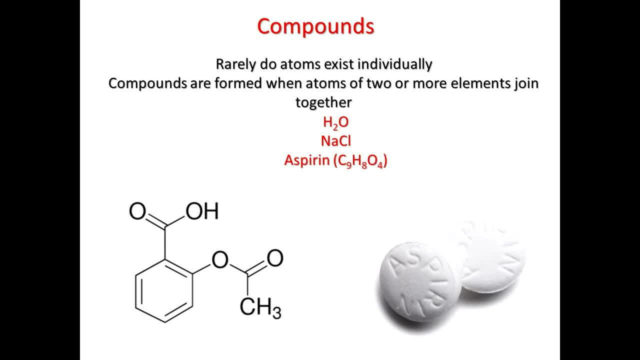 of course N-acid. So we've already talked about sodium chloride, which is, of course, N-acid, So we've already talked about sodium chloride, which is, of course, N-acid, N-acl. Second example, of course, is H2O, So in other words, two hydrogen atoms and an oxygen. 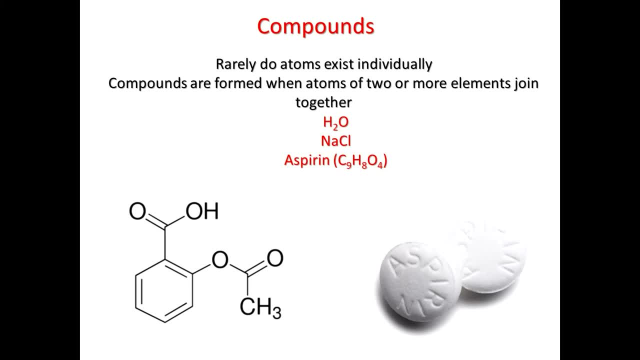 atom. They're really ions, but that's for another day. Combine in a two-to-one ratio to give you water, And of course, water is incredibly important to all of us. Without water we would not exist. of course, Again, similarly to the previous example of glucose, if you were to. 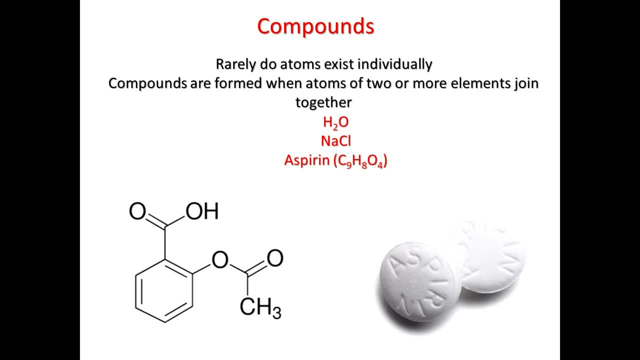 combine, in this case, nine carbons, eight protons, or eight hydrogens, I should say, and eight oxygens in there and put them together. you would have a two-to-one ratio to give you water. Put them in this arrangement And this is simply aspirin, which of course is a medicine that we 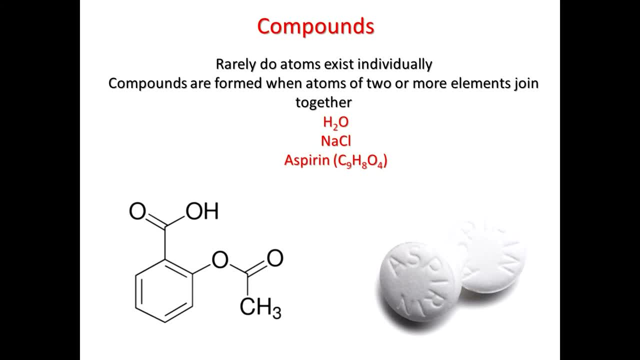 take for headache relief, And of course, it's actually used to thin the blood for some patients as well nowadays. So in other words, this should show you the huge scope of chemistry. Just by simply combining different elements in different ratios, you can form really interesting. 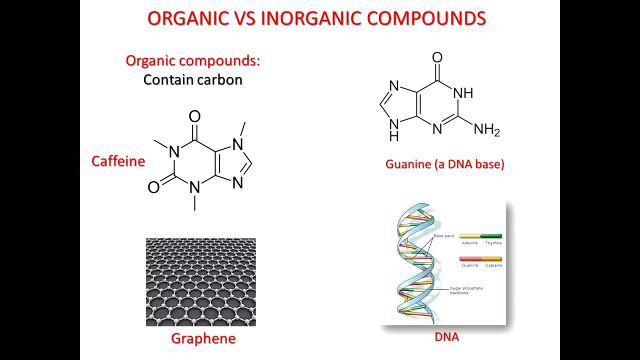 materials. So what is an organic compound and what is an inorganic compound? Well, on the top left we have an organic compound, which is caffeine. Now, organic compounds contain carbon atoms. okay, So anything containing a carbon atom you could call an organic compound. 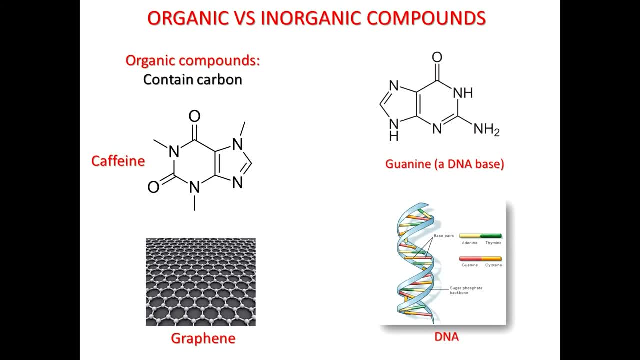 So caffeine? I don't know about you guys, but I love coffee. It's fantastic, And, of course, caffeine is the major sort of chemical in coffee that gives you that alertness, And so it's a very special chemical for a lot of people. 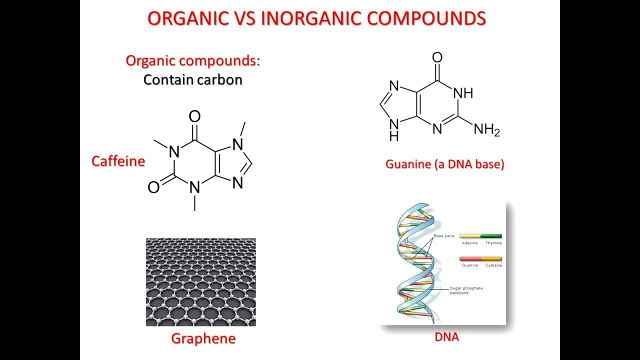 Underneath you'll see graphite. Now this is similar to graphite, which is a lump of coal essentially, but this is graphene, which is essentially made of carbon atoms linked together in a sort of hexagonal, sort of chicken wire arrangement, And this is a truly two-dimensional material And it's the 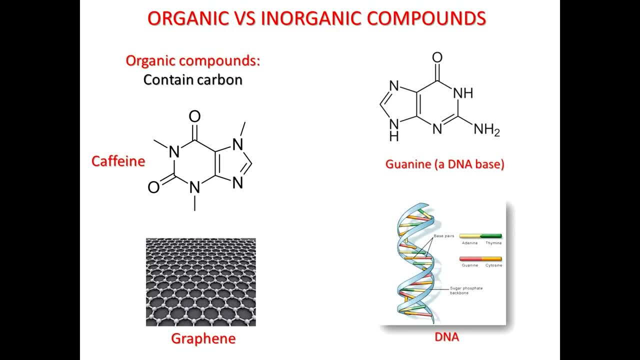 first two-dimensional material And this is incredibly important for many reasons. It's got massive applications in all sorts of things because it's incredibly light and it's incredibly strong conductive. It can do all sorts. It's been used, for instance, to filter water up to a high quality. 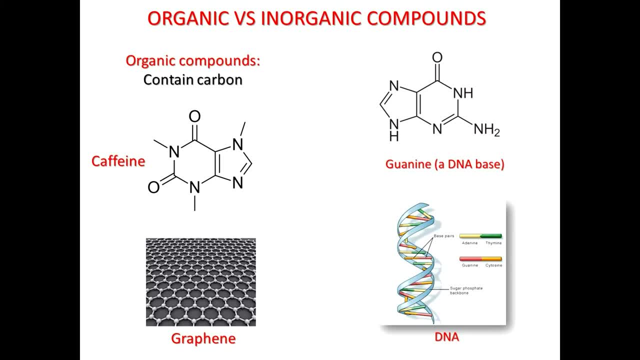 to drinking level just by passing water through it, And it's used in things like the new type of light bulbs, for instance, And it really is the wonder material nowadays. So have a look at that in the literature. Likewise, if you look on the top right, we've got guanine, which is again 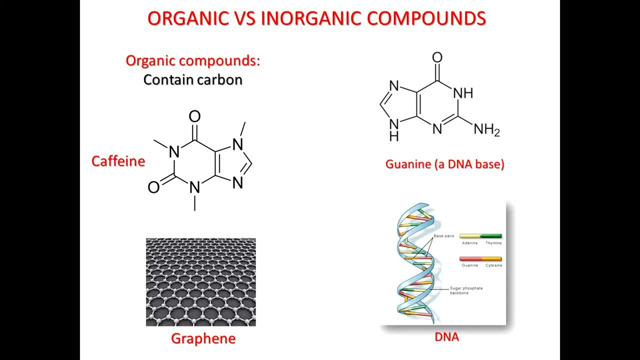 it looks similar to caffeine, but it's very different. It's actually a DNA base, okay? So in other words, this molecule is a DNA base, So it's a DNA base, So it's a DNA base, So it's a DNA base. 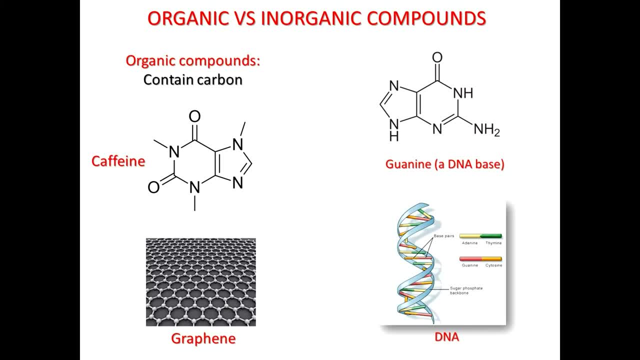 This molecule is one of the molecules that are found right in the middle of DNA. okay, And of course, DNA is essentially the material or the information carrier in our bodies, And so, essentially, it allows life to happen and it allows us to maintain life. So the importance: 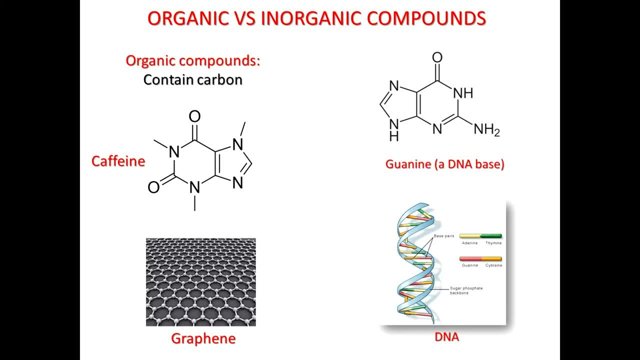 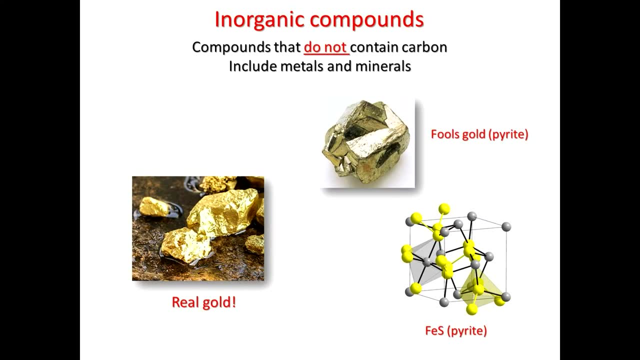 of guanine cannot be overemphasized, of course. So these are organic molecules, So of course they're very, very interesting and important. Inorganic materials are also important. Essentially, these are materials that do not contain carbon, okay, And so these will include metals. So, for instance, on the left-hand side. 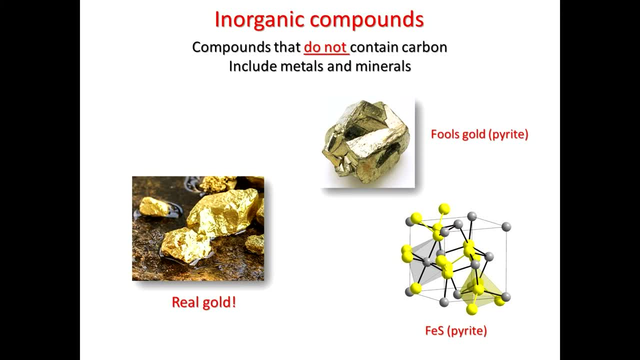 here I've got real gold And so essentially, if anyone who's watched Gold Divers on Discovery Channel will know that it's fantastic, You can find it. If you dig deep enough and dig hard enough and clever enough for it, you can find nuggets of gold. So some people actually dive. 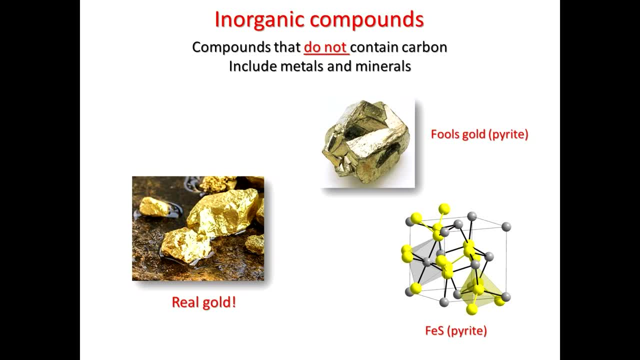 to the bottom of the seabed to do this- Very dangerous of course, And it's worth a lot of money. On the right-hand side- so that's essentially that's made up of gold atoms linked together, So nothing but gold atoms. On the right-hand side, however, is something called 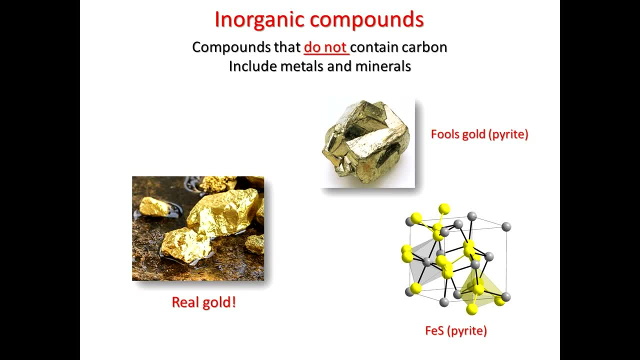 pyrite, which is fool's gold, because basically it's not gold but it looks like gold, And so on. the bottom right is the actual unit cell, And I'll tell you about a unit cell in a second, but essentially it's the unit cell of pyrite. The gray spheres are the sulfite or the sulfur. 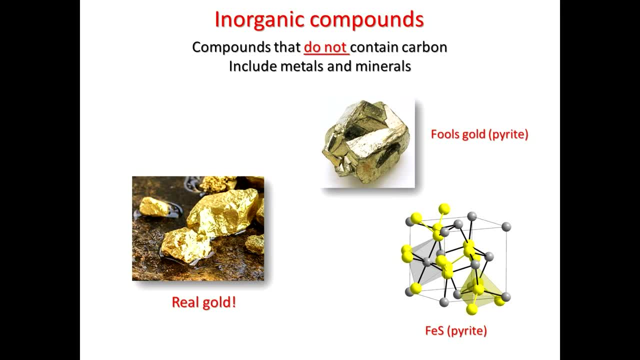 atoms, or ions, I should say, And the yellow spheres are the iron ones, And, essentially, if you connect them in this particular way, or when they connect in this particular way, they form a mineral called pyrite or called fool's gold sometimes. okay. 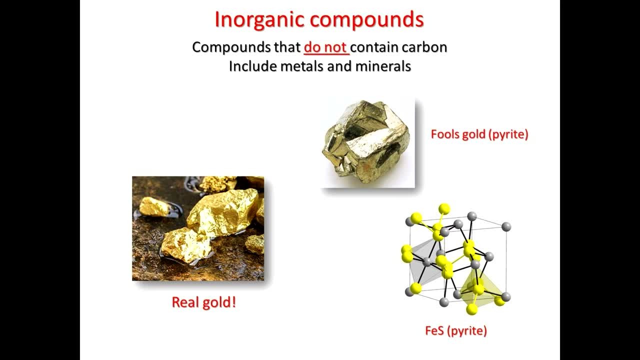 A unit cell essentially is, by the way, is just a imagine. this is a sugar cube, okay, And then just imagine that the real material, the whole big bulk material that you find pictured above, it is essentially lots of those sugar cubes arranged into the packet.